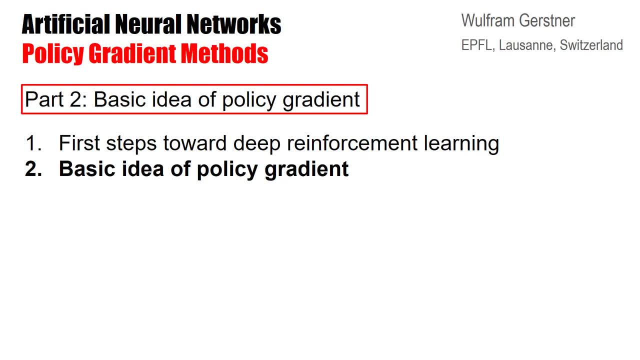 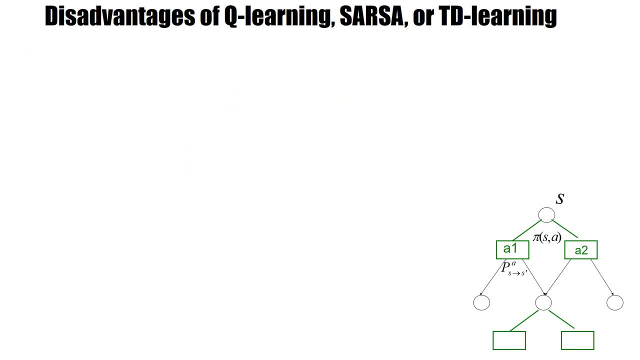 Welcome to the lecture series on policy gradient methods. In this video I present the basic idea of policy gradient. We are all familiar with TD methods, such as Q-learning or SAGSA. They start from a discrete graph with states s another state s prime that are connected by actions. 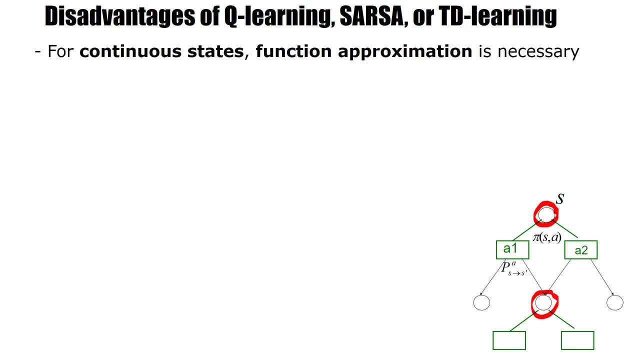 There are transition probabilities Now for continuous states. Q-learning is no longer that good because function approximation is necessary. You may say: function approximation, what's the problem? You just take your neural network, it's a great function approximator. Well, it turns out it's potentially unstable. 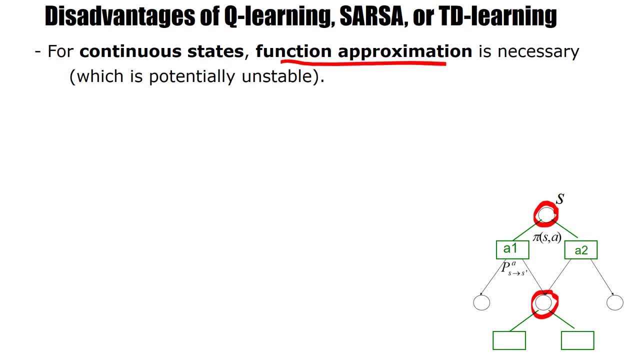 because if you change with a function approximator, if you change the weights of the network, it's going to be unstable. If you change the weights of the network, it's going to be unstable. If you change the weights of the network, it's going to be unstable. 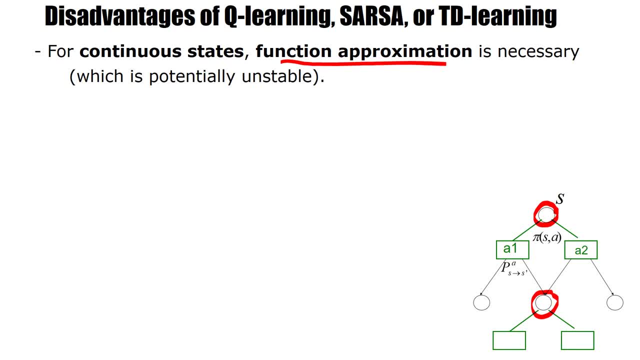 If you change the weights of the network, if you change the parameters, then you always change also neighboring states. This might be good for generalization but it might do the wrong generalization and that makes it unstable. Now, even in fully observable Markov settings, these kind of discrete settings like on the graph. 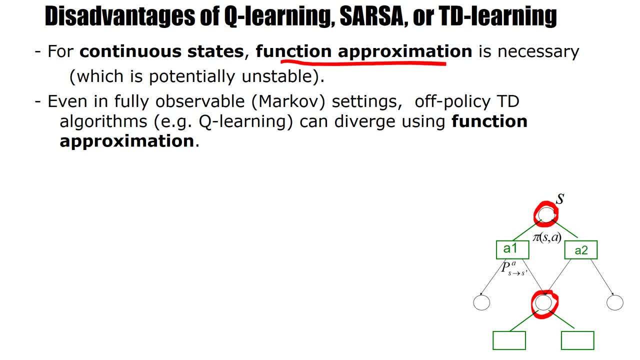 off-policy. TD methods like Q-learning can diverge. using function approximation- Again, because function approximator links, states that maybe should not be linked. it's not necessarily stable. It gets worse if you have partially observable environments. that means non-Markovian. 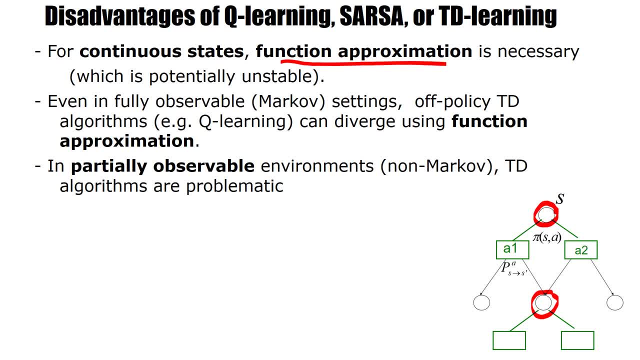 You cannot distinguish two states just from the present observation. Then TD-learning algorithms become really problematic. Then TD-learning algorithms become really problematic, And while previously I've talked about continuous states, it even gets worse if you have continuous actions. Well, the source of all these problems is: 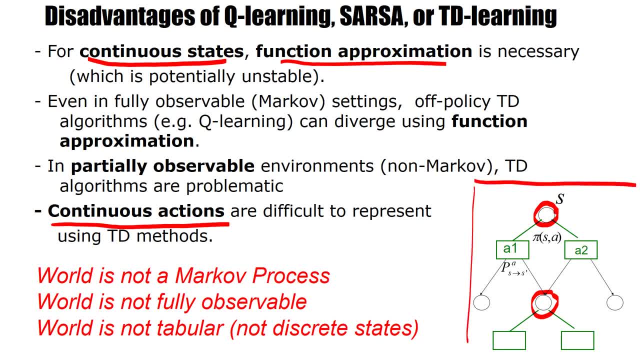 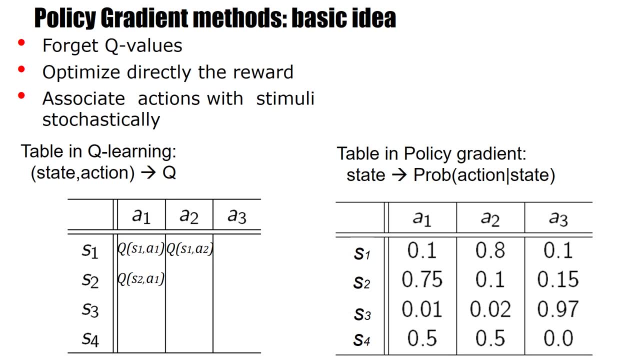 that the world is not a Markov process of this type. The world is not fully observable and the world is not tabular, It's not just existing of discrete states. So with policy graded methods, the basic idea is that we forget about Q values. 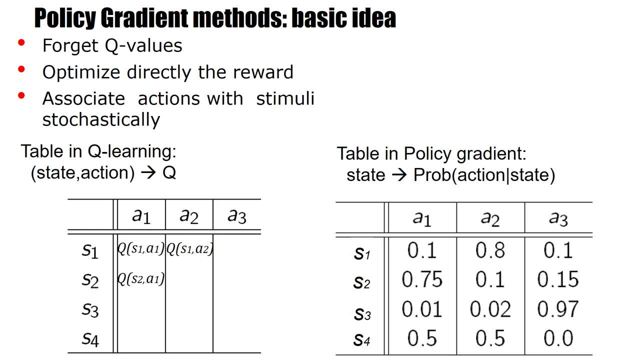 We optimize directly the reward. We associated actions with stimuli stochastically. So let me just compare the two philosophies In Q learning. we build a table. For each state action pair we assign a Q value, And so, for example, for state two and action one, 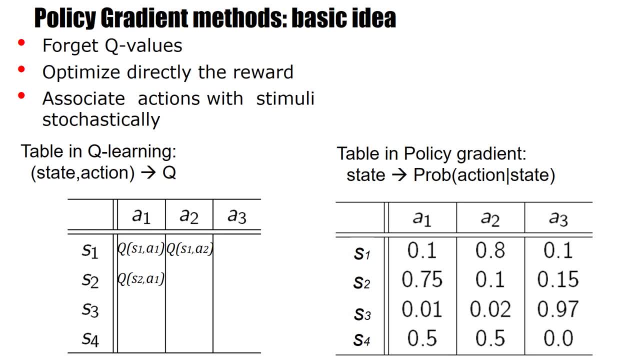 we have a Q value, Q of S two and action one, And then, with this Q value, we play around, We use Epsilon, greedy or we use softmax methods to choose the best actions to build a policy. Now, instead, we can have a table in policy gradient. 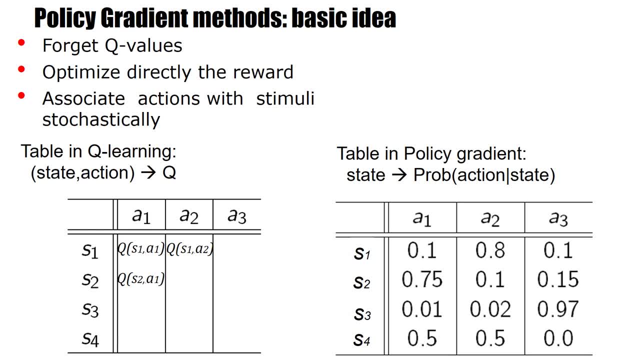 that says we directly associate each state action pair. So we have a table in policy gradient that says we directly associate each state action pair. So we have a table in policy gradient that says we directly associate each state action pair. So we have the probability of a state. 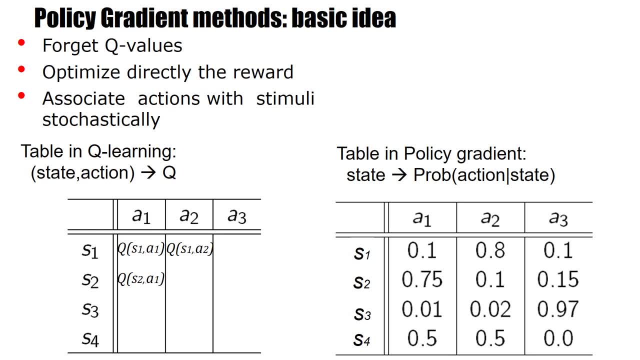 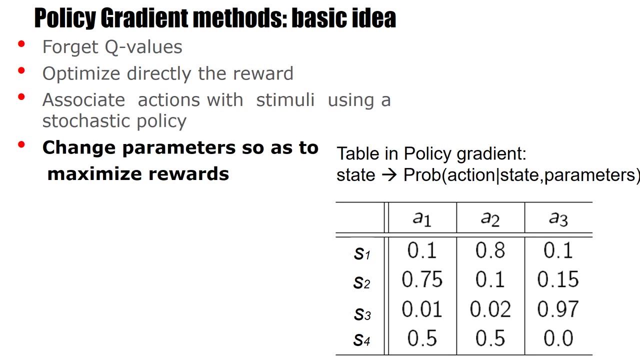 with a probability of action giving a state. So for example, again I'm in state two, I have three actions, and the three actions together are taken with certain probabilities, And the only condition is that these probabilities must sum to one. And now the idea is that these table entries 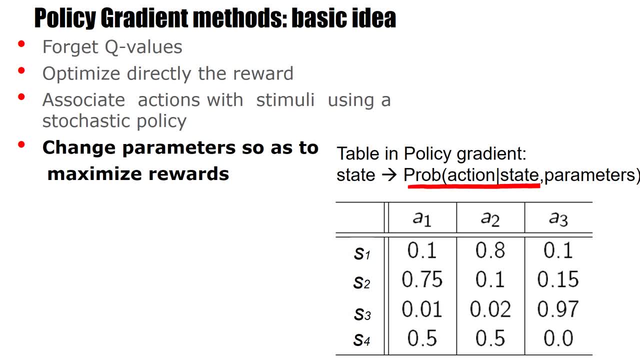 these probabilities of action given a state will actually will actually depend on parameters, And so now we change the parameters so as to maximize the rewards. So we can write this stochastic policy: The action depends on the state and it also depends on parameters. So what you'd really show in this table over here is this stochastic policy. 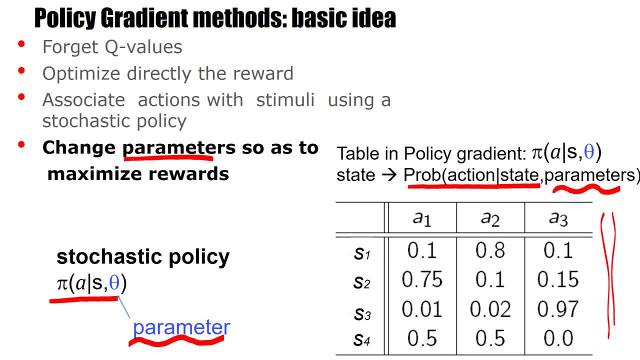 P for an action given the state. And all this depends on parameters. So I write here the parameters explicitly in terms of an entry in this function. here You could also write it in that form: P of A given S, And then the whole thing depends on parameters, And these parameters 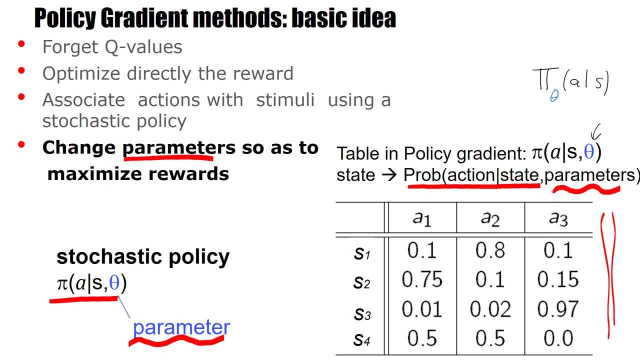 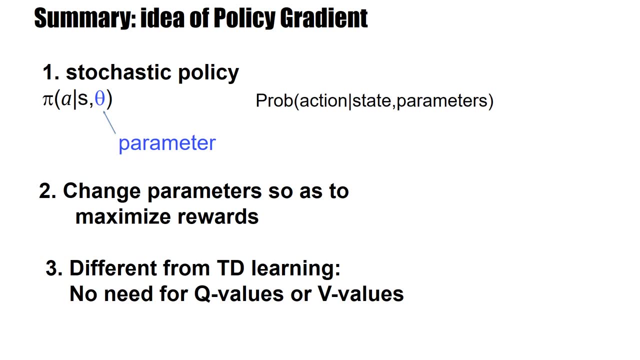 I could also write as an index down here. It's just two different notations And in both cases it's really the same thing. So just to summarize this basic idea of policy gradient: we have a stochastic policy. It's denoted as a policy P that depends on parameters. So if the policy is 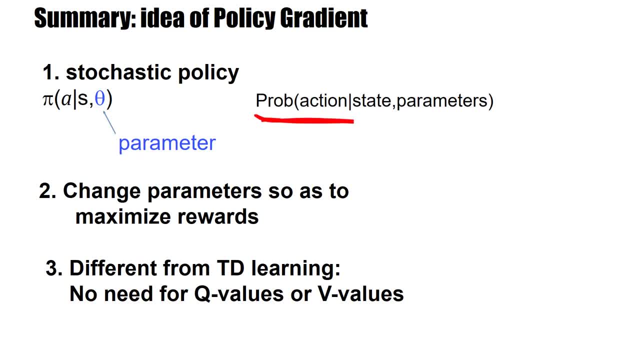 directly the probability of the action given by the state. then the policy P is the same as the policy of taking an action in a certain state, And then we change these parameters, such as to maximize the rewards. And what's different from TD learning? there is no need for any Q values or V. values. 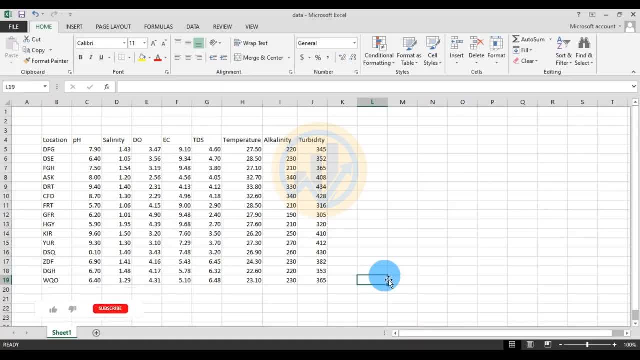 Hi everyone, welcome to statistics bios of an YouTube channel. Today we will discuss topic how to analyze it in the principal compound analysis in arginbrow software. The data already entered in the excel sheet, The first one for the location, the 15 location we take. 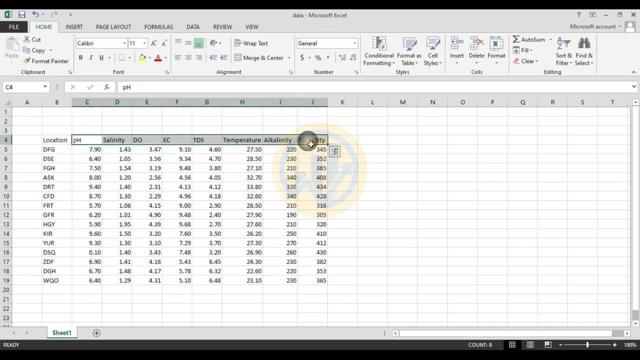 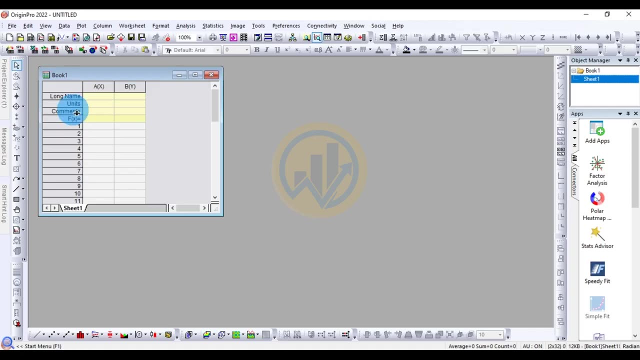 and the 8 the water parameters: the pH, salinity, DO, EC, DDS, temperature, alkalinity and the temperature. The data copy paste to the arginbrow software. First copy the location and water parameter title copy. go to the arginbrow software. the paste. Okay. next to the data. 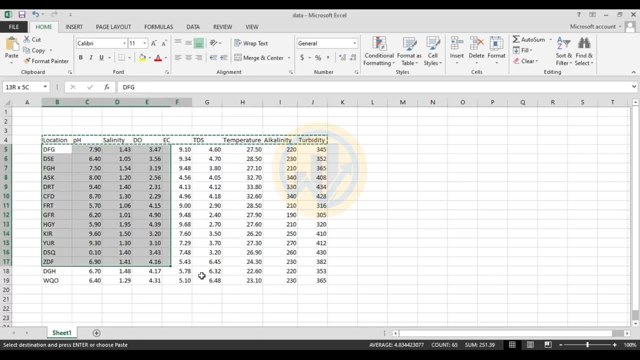 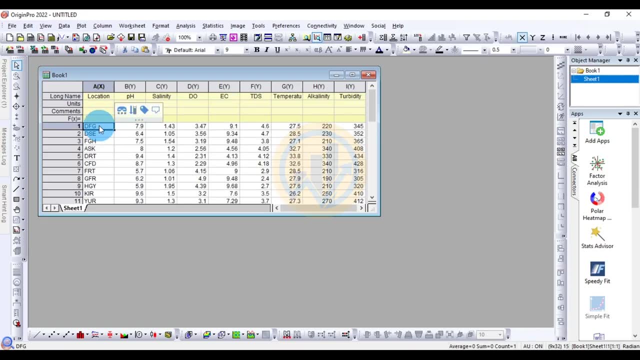 copy. copy the data, go to the arginbrow software and paste it. Okay, the next go to the. for the statistical menu: the statistics, the multivariated analysis. the first one for the sub menu, the principal- compound analysis. the first one for the sub menu, the principal. 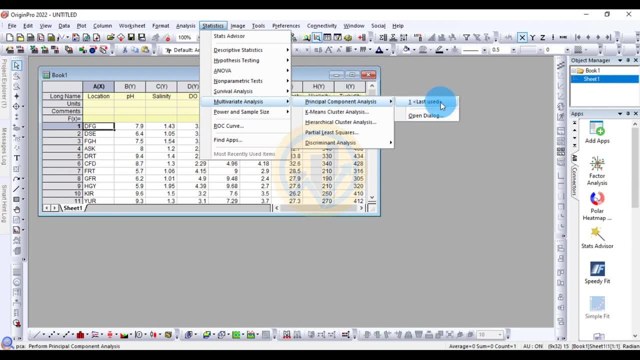 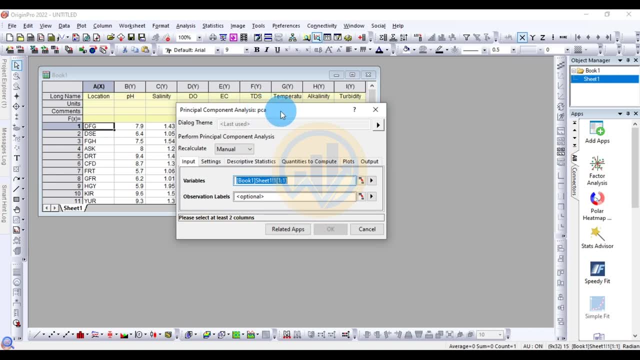 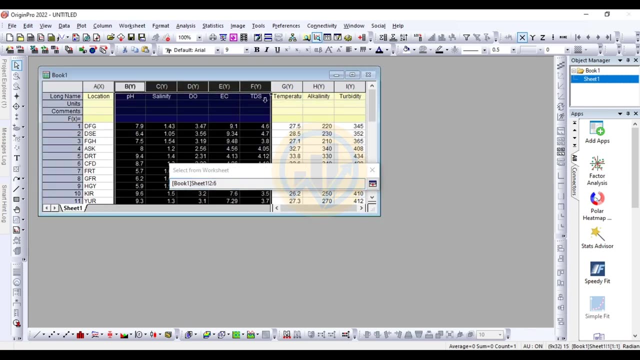 compound analysis. then click the last used, The open the new tab for the principal compound analysis, the PCA. the first one for the input, the variable. select the water parameter, the- we select the 8 water parameter pH to turbinity. The next one for the observation level for: